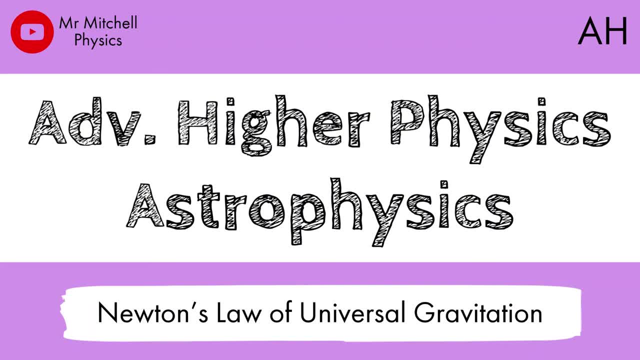 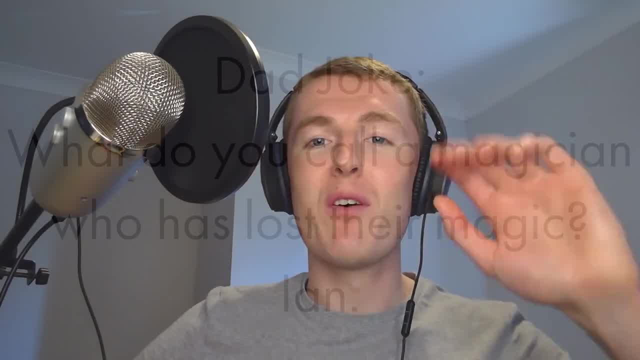 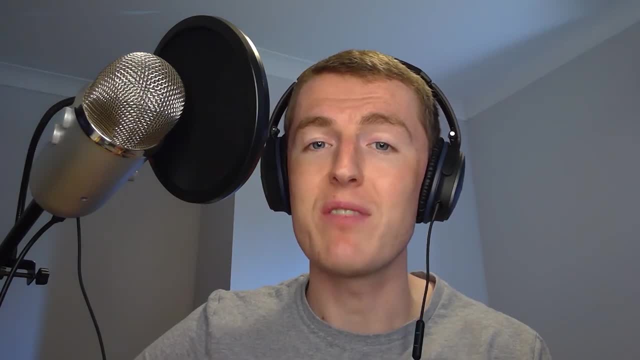 Hey folks, welcome back. In this video we're going to go over three worked examples to show you how to do problems involving Newton's law of universal gravitation. Now, if you haven't already done so, check out my previous video covering the theory on this topic, and that way you can apply what you 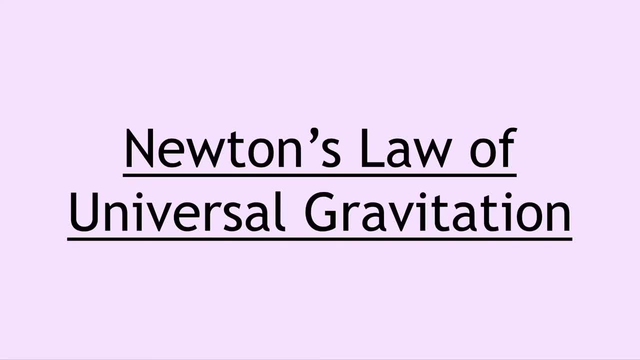 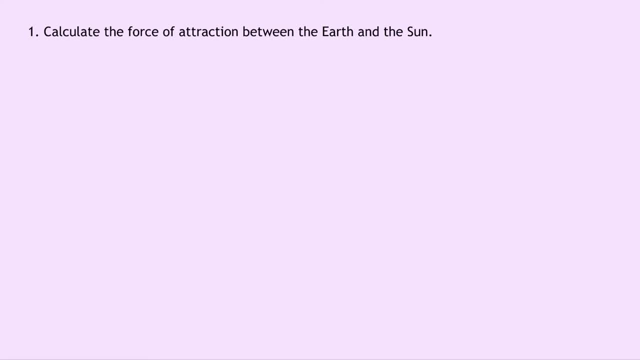 learned in that video to this one. So let's get started Now. this is a bit of recap from the higher physics course, because Newton's law of universal gravitation was seen there. Question one says: to calculate the force of attraction between the earth and the sun, 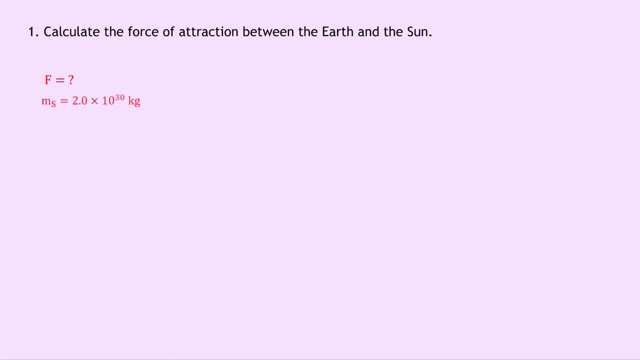 Well, writing down what we know from the question, we're trying to find the force f. We know the mass of the sun is 2.0 times 10 to the 30 kilograms, so I'm going to call that m subscript s. The mass of the earth, which we'll call m subscript e, is 6.0 times 10 to the 24. 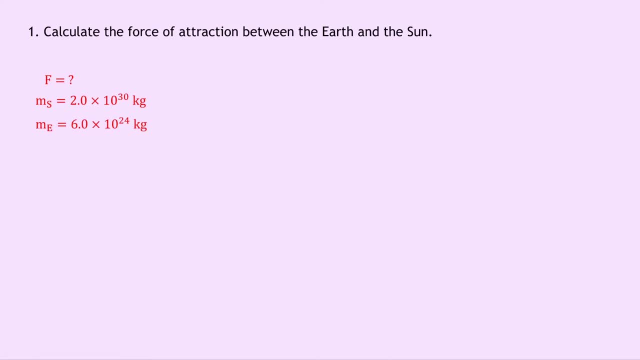 kilograms and you get both of these on the data sheet in your exam. The universal constant of gravitation g is 6.67 times 10 to the minus 11 meters cubed per kilogram per second squared, and the distance r between the earth and the sun is: 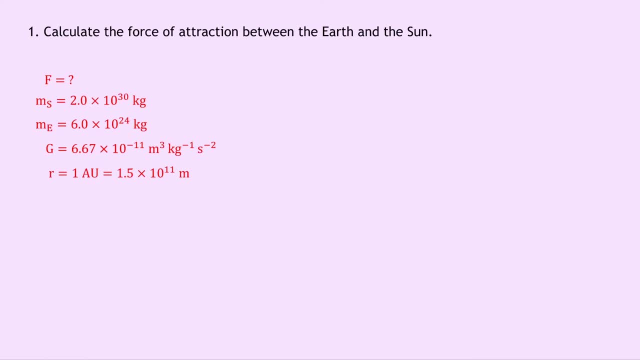 1 au, which is the same as 1.5 times 10, to the 11 meters. Now, just to point out, you get all four of these values on the data sheet in your exam. So writing down the equation for Newton's law of: 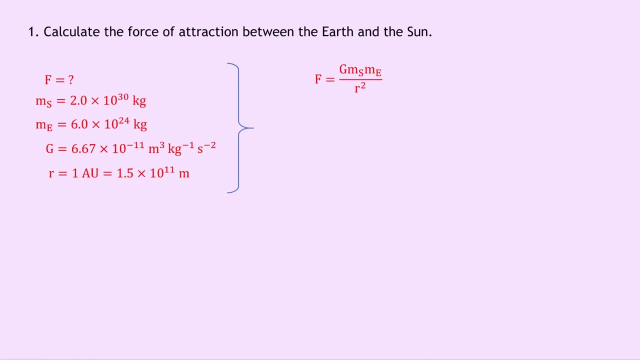 universal gravitation. we have f equals gms, me over r squared. so instead of using ones and twos, we're just using s and e to represent the sun and earth. Substituting in our numbers, now we get 6.67 times 10 to the minus, 11 times 2.0 times 10 to the 30 times the 6.0 times 10 to the 24 divided by 1.5. 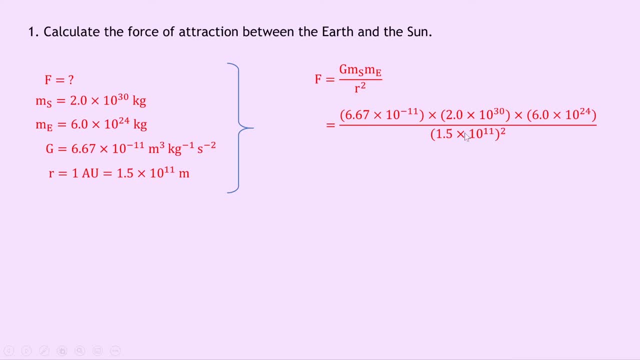 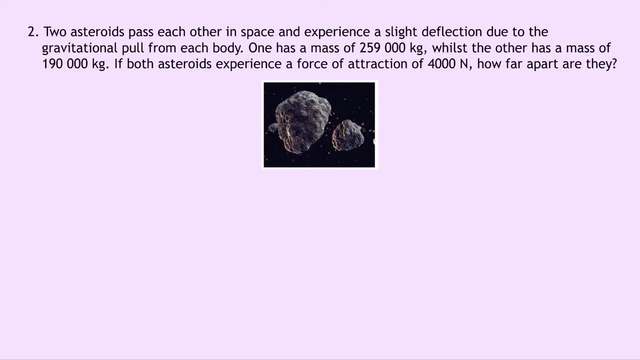 times 10 to the 11 squared. So make sure you square that term there And putting that into your calculator should give you an answer of 3.6 times 10 to the 22 newtons. Question two says that two asteroids pass each other in space and experience a slight deflection due to the 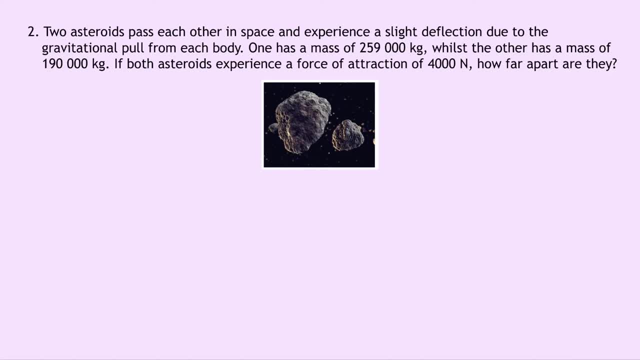 gravitational pull from each body. One has a mass of 259,000 kilograms, whilst the other has a mass of 190,000 kilograms. If both asteroids experience a force of attraction of 4,000 newtons, how far apart are they? Well, writing down what we know from the question, we'll be able to find out the 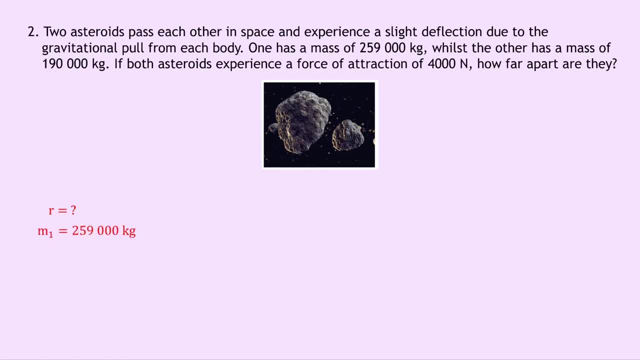 question we're trying to find are: we know the mass m1 is 259,000 kilograms and mass m2 is 190,000 kilograms. We also know the universal constant of gravitation g is 6.67 times 10 to the minus 11. 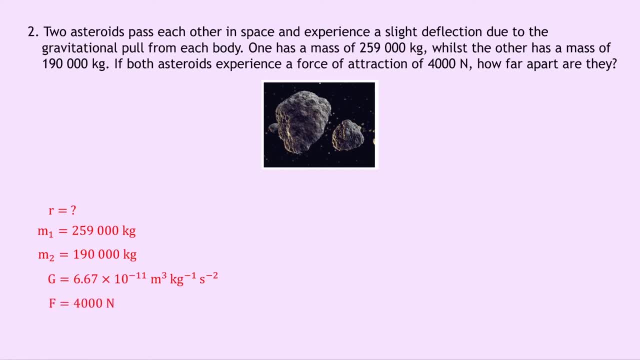 meters cubed, per kilogram, per second squared, and the force we're told is 4,000 newtons. So, writing down our equation, we have f equals gm1 m2 over r squared and substituting in the numbers now we get 4,000 equals 6.67 times 10 to the minus 11 times 259,000 times 190,000.. 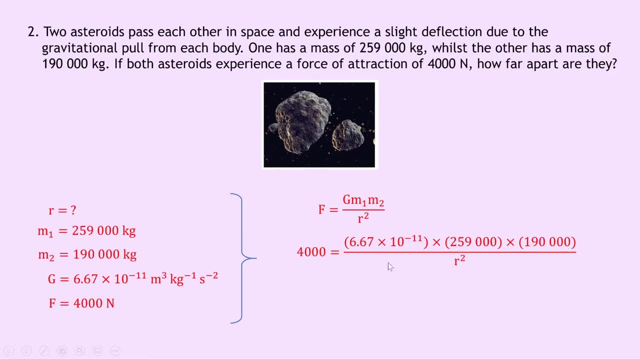 Now we want r squared on its own on the left hand side. so right now it's on the denominator of this fraction, so we can cross multiply it with this side to get it on its own on this side. So if we do that, we swap the 4,000 and the r squared so that r squared equals this whole term divided by 4,000. 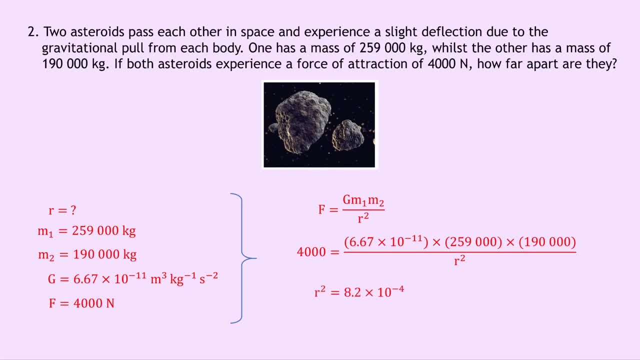 and if you put that into your calculator you should get r squared equals 8.2 times 10 to the minus 4, and then taking the square root of both sides gives an answer of r equals 0.03 meters, or in other words three centimeters. 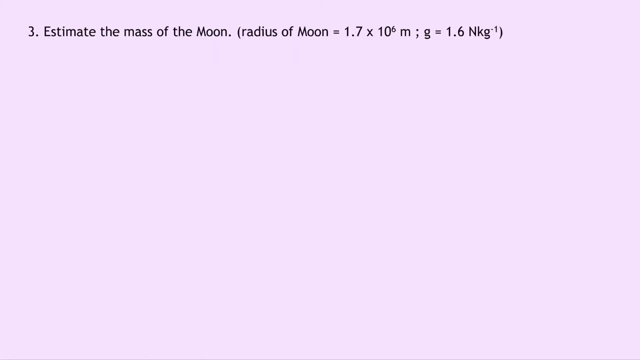 So the asteroids are in fact very close together. Lastly, question three is to estimate the mass of the moon. and it tells us some data about the moon because it doesn't give us that on the data sheet in the exam. So the radius of the moon is 1.7 times 10 to the 6 meters and the gravitational 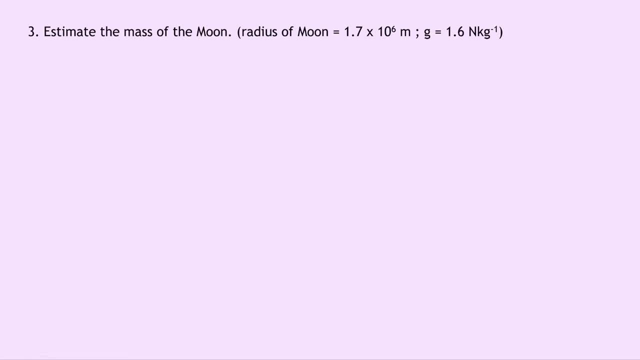 field strength g on the moon is 1.6 newtons per kilogram. So what we need to do first of all is consider an object of mass m placed on the surface of the moon. The gravitational force of attraction between the two can be represented by both f equals mg. remember, that's just a form of f equals. 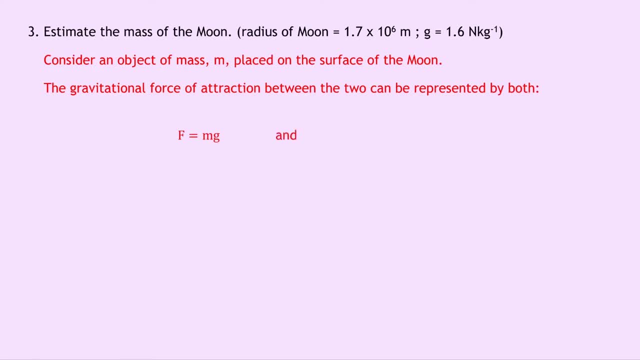 ma or w equals mg and the other equation for force, which is f equals g, subscript m, m over rm squared, where the subscript capital m there represents the moon and the small m is just our mass of the object that we've placed on the surface of the moon. So because we've got two, 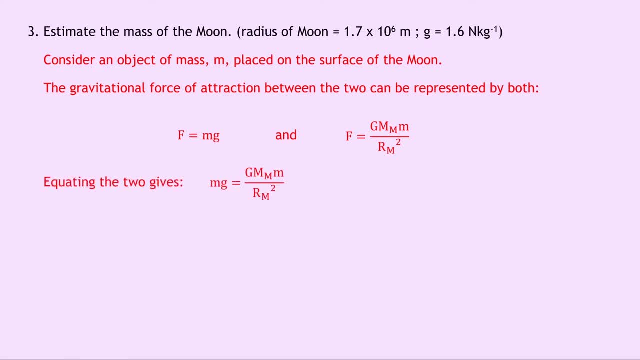 expressions for the force equating the two gives us. mg is equal to gm, subscript m, m over rm squared. and now cancelling the m's from both sides because we've got an m there and an m there, and rearranging for m, subscript m, the mass of the moon which we're trying to find, we get.